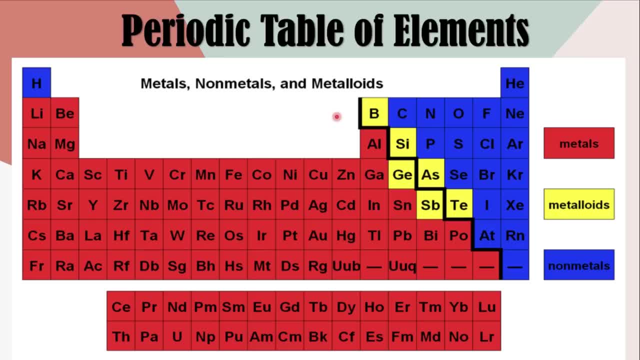 Shown in your screen right now is the periodic table of elements, which are grouped as to metals, metalloids and non-metals. Metals are those colored with red, Metalloids are yellow And non-metals are blue. 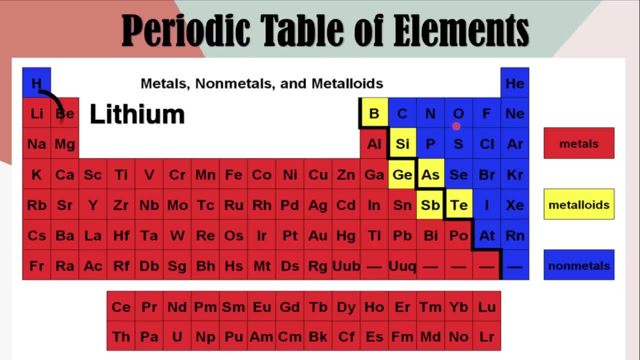 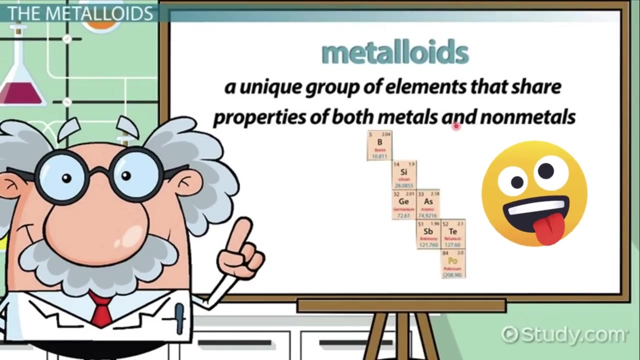 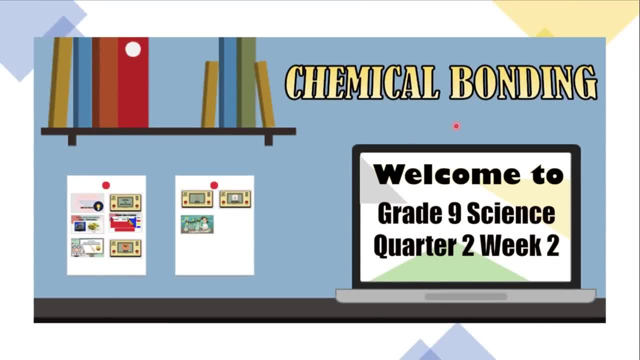 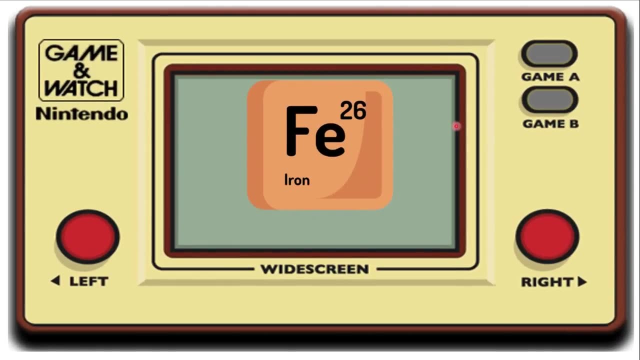 So as easy as that, Let us start with our activity. All you need to do is identify if the element is metal or non-metal. First one, iron. By looking in your periodic table of elements, iron is a metal element. That's correct. 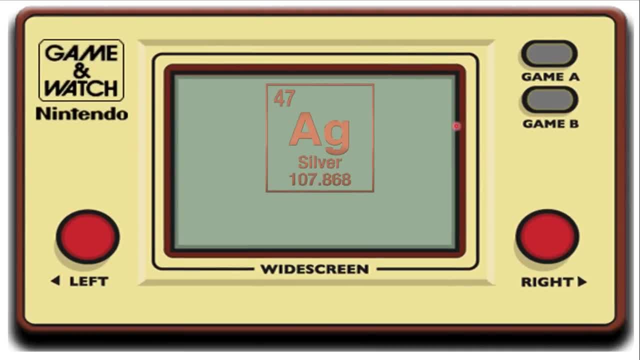 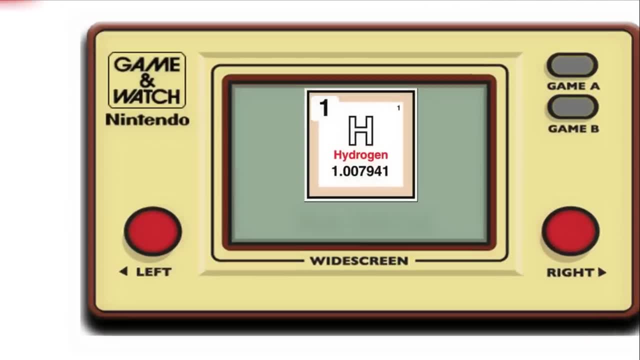 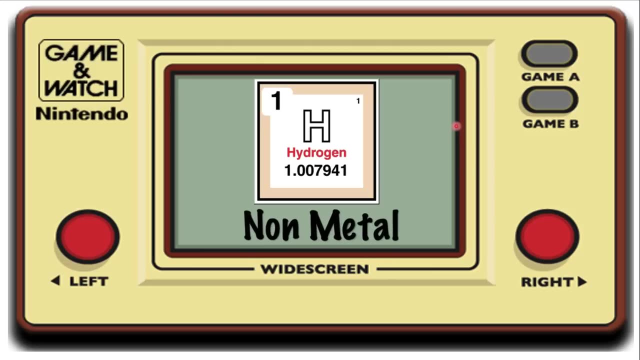 Next silver, Next copper, Silver, Silver, Silver, Silver, Silver, Silver Silver is a metal element. That is right. The last one, hydrogen. Hydrogen is an example of a non-metal element. Good work, class. 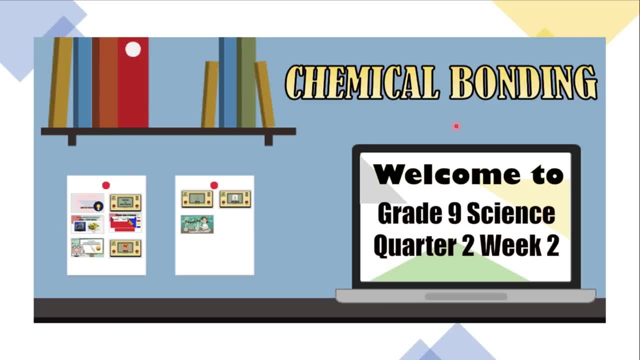 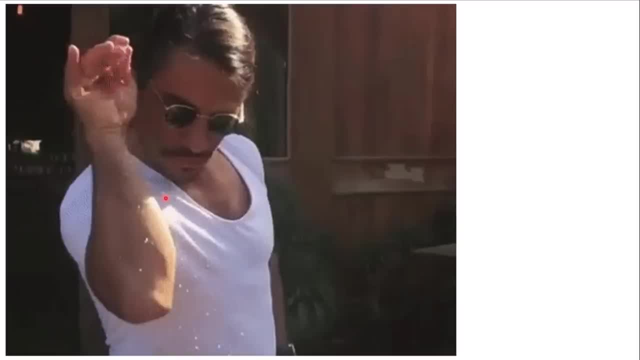 Now let us proceed with our lesson for today. Do you know this man? He is the famous chef called Salt Bae. He is popular because of his way of pouring salt. Now, do you know that table salt is an example of compounds? 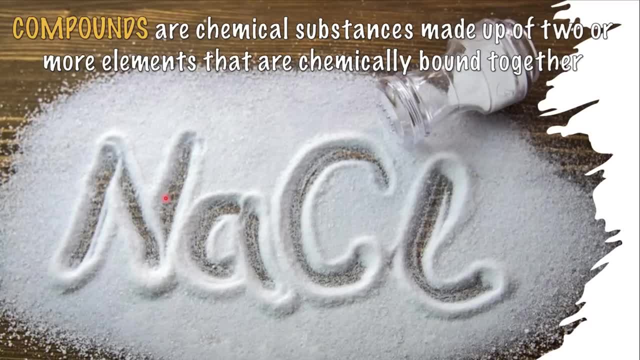 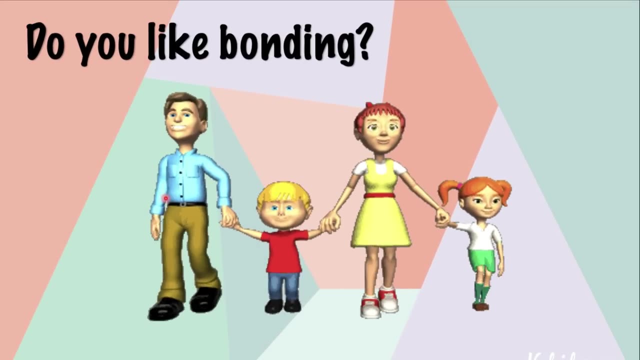 Compounds are chemical substances made up of two or more elements that are chemically bound together. One good example is salt, Sodium chloride or the table salt. Do you like bonding with your friends, family or loved ones? Do you miss bonding with your classmates? 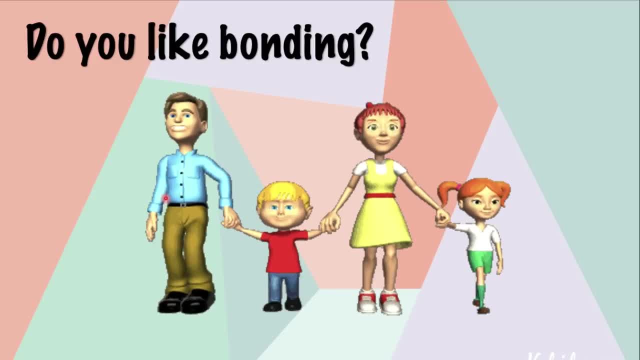 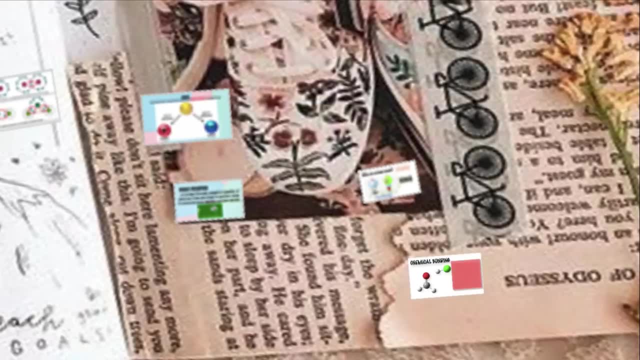 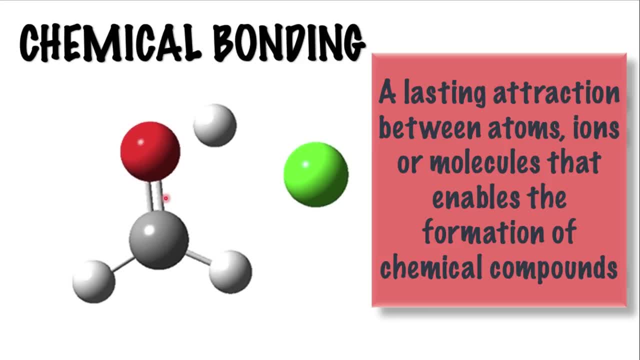 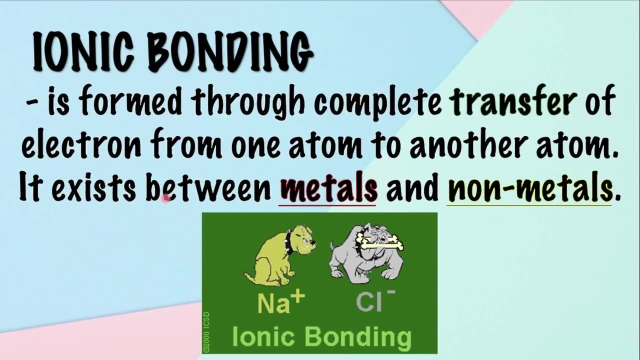 There is a lasting attraction between atoms, ions or molecules. that enables the formation of chemical compounds, And there are several types of chemical bonding. One type is ionic bonding. It is formed through complete transfer of electron from one atom to another atom. 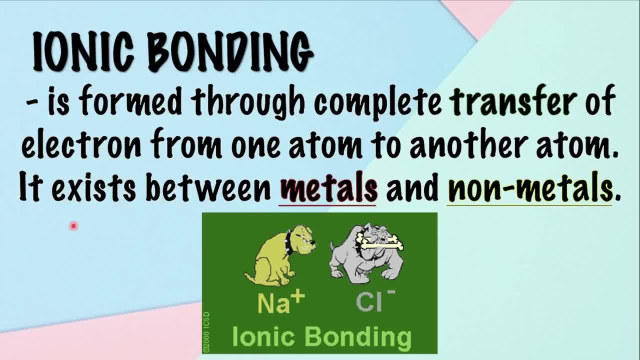 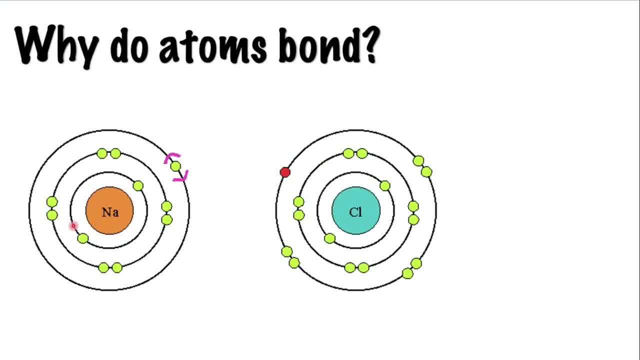 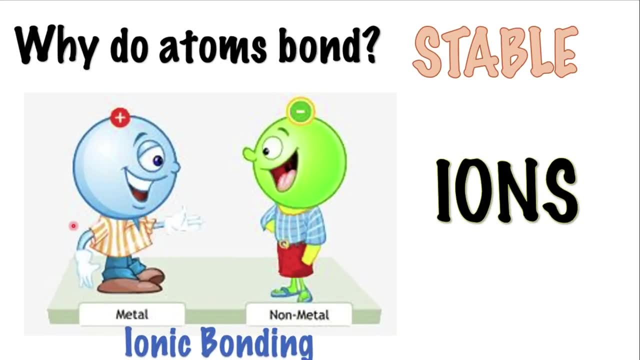 It exists between metals and non-metals. Now the question is: why do atoms bond? Atoms bond to become stable. When a metal element bond with a non-metal element, that is ionic bonding, Wherein ions are formed. 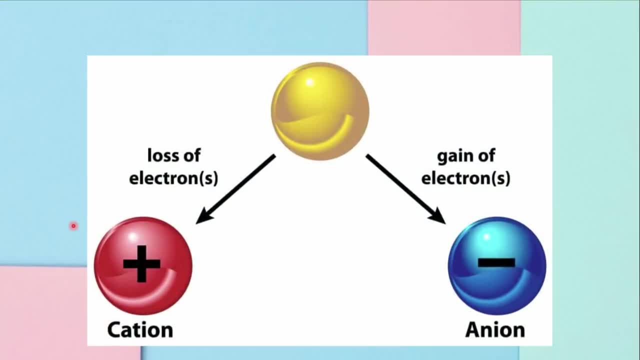 Ions are formed. Ion is an atom or molecule with positive or negative charge. It is formed after a metal atom transfers its valence electrons to non-metals. It is formed after a metal atom transfers its valence electrons to non-metals. 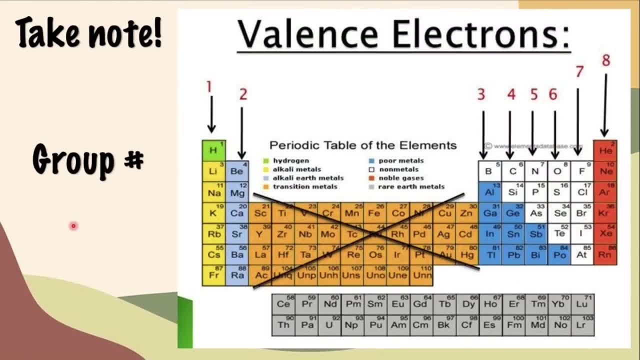 Take note: class valence electron is the electron found in the outermost shell of an atom. You can determine the number of valence electron by looking at its group number in the periodic table of elements, For example. For example, Oxygen is in group 6, that is why its valence electrons is 6.. 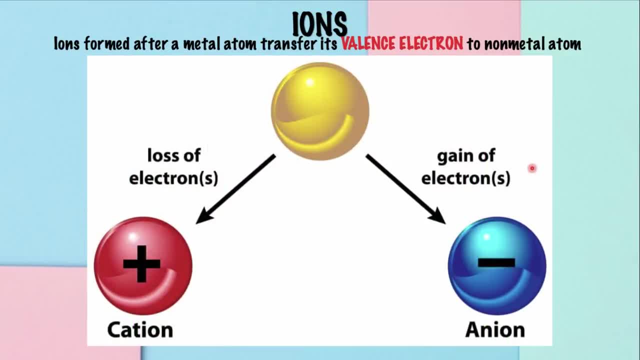 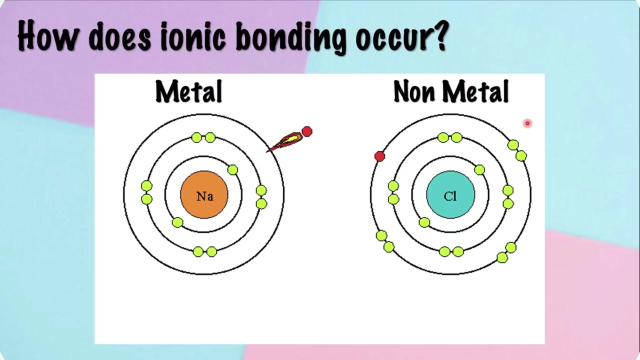 Next, ions are classified as cation and anion: Cation when a metal atom loses electron. Anion when a non-metal atom gains electron. Are we clear class? Now let us proceed. Just like what I said earlier, it happens between a metal and non-metal element. 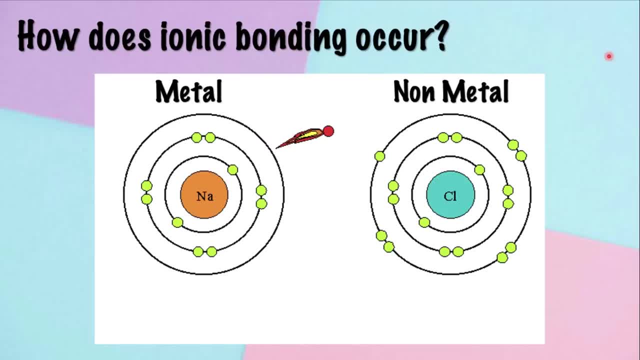 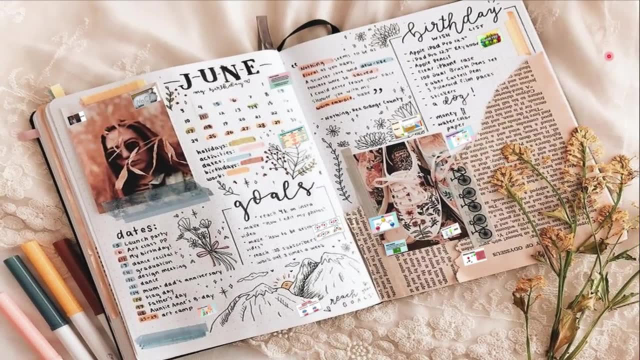 If there is a complete transfer and gaining of electrons, ionic bonding happens. One example is sodium chloride, wherein sodium is metal and chlorine is non-metal. Next type of chloride, The chemical bonding that we are going to have is covalent bonding. 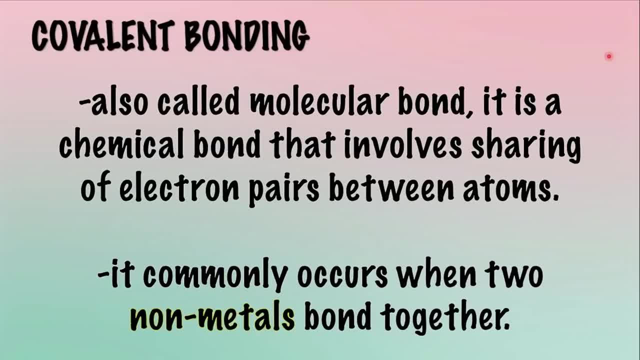 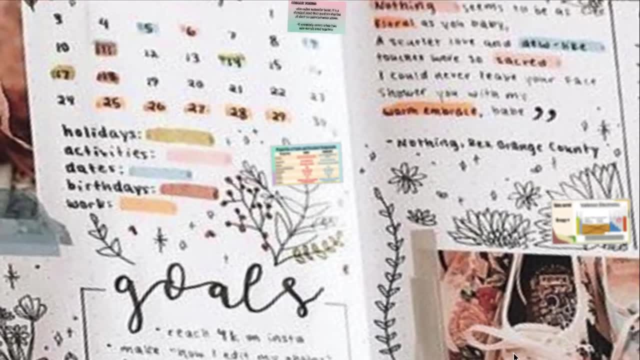 Covalent bonding is also called molecular bond. It is a chemical bond that involves sharing of electron pairs between atoms. It commonly occurs when two non-metals bond together. Non-metals have strong energy attractions. Non-metals have strong energy attractions or high electron numbers. 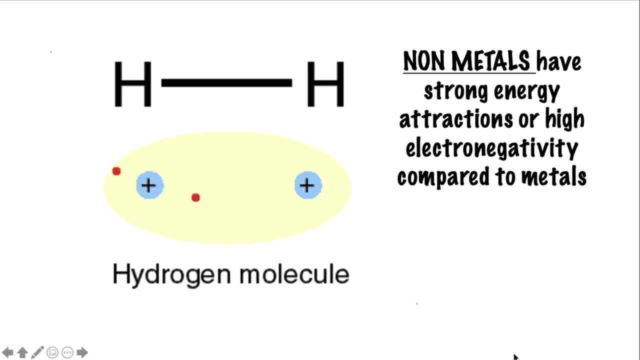 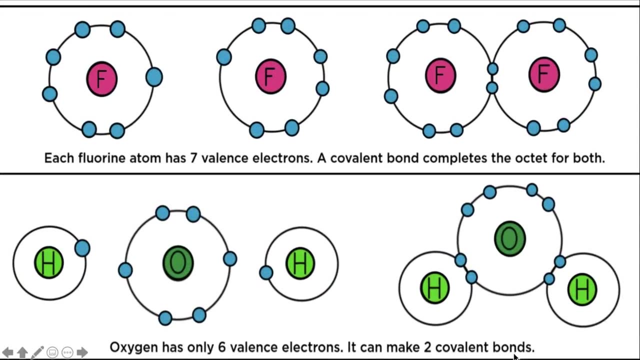 They have strong electronegativity compared to metals, just like hydrogen. They do not need to give electrons to be stable. Instead, they gain or share electrons to obtain stability. For example, fluorine is a non-metal element. Covalent bond completes the octet for both. 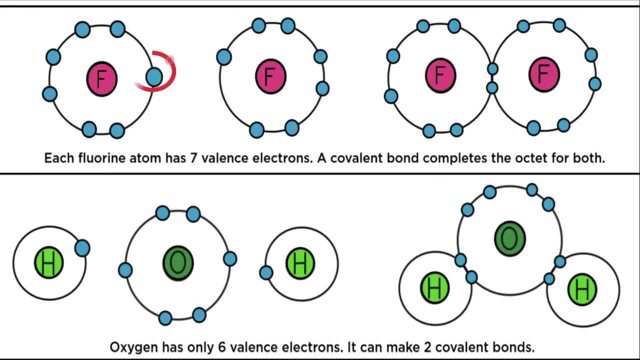 Sharing of electrons will obtain stability. Another one is Oxygen, a non-metal element that has six valence electrons. It can make two covalent bonds with hydrogen, which has one valence electron, resulting to H2O or water That is covalent bonding. 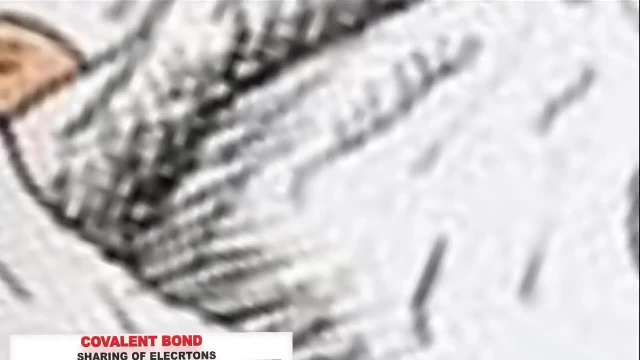 Covalent bonding. There are two types of covalent bonding. There are two types of covalent bonding. There are two types of covalent bonding: Non-polar covalent bonding. Non-polar covalent bonding. Non-polar covalent bonding. 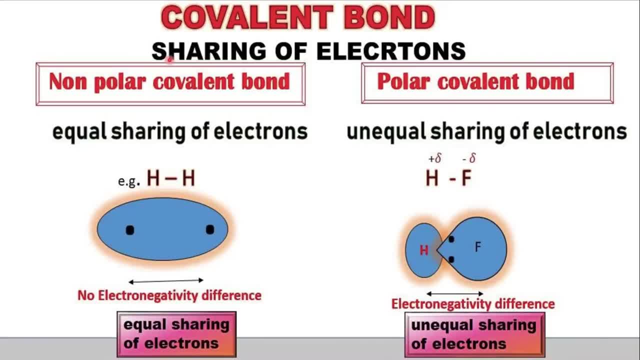 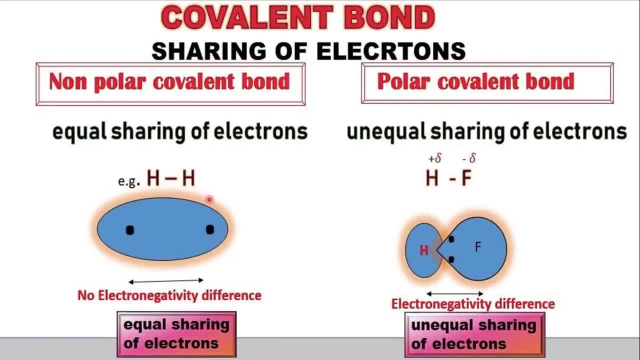 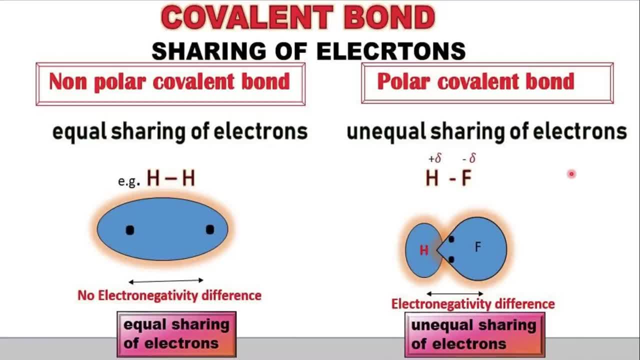 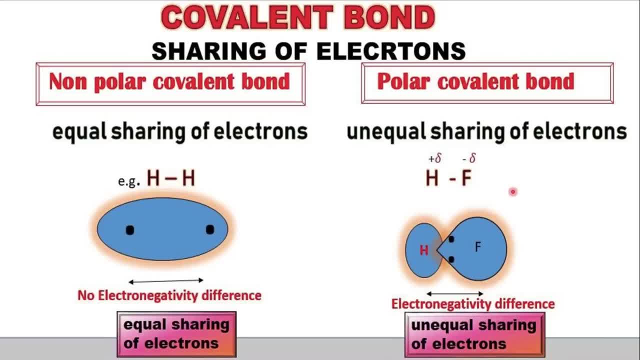 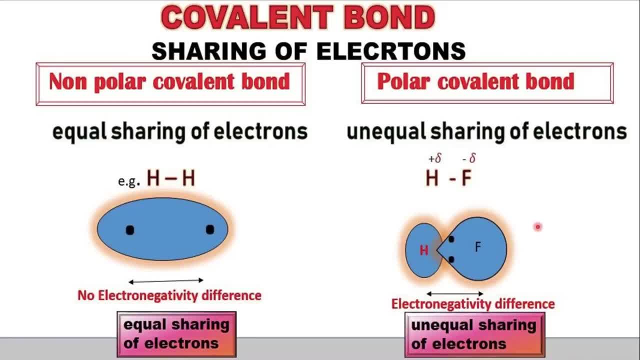 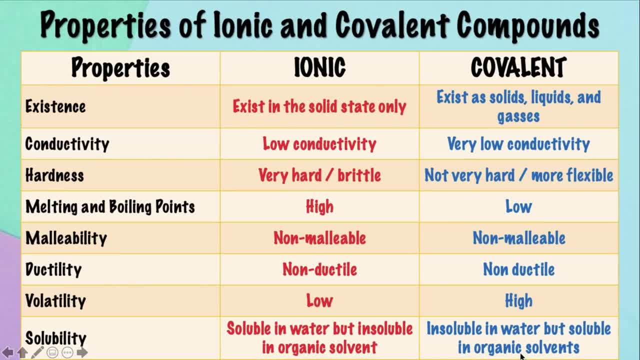 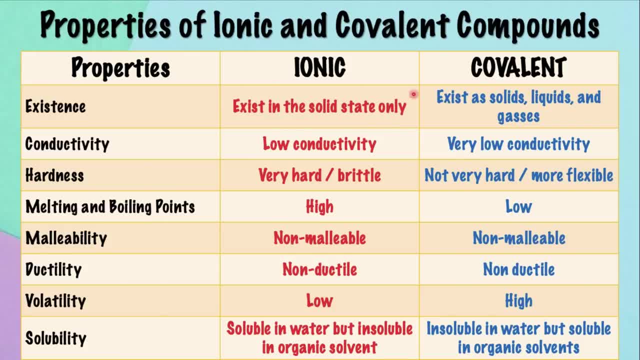 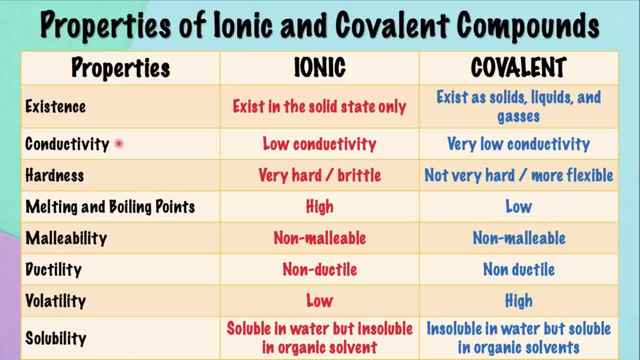 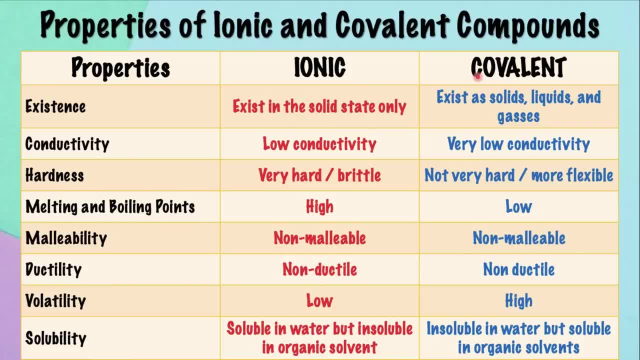 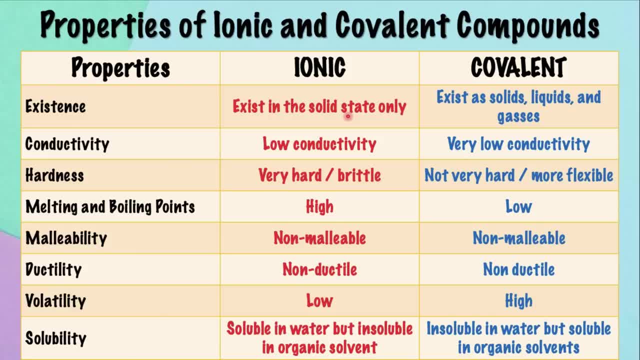 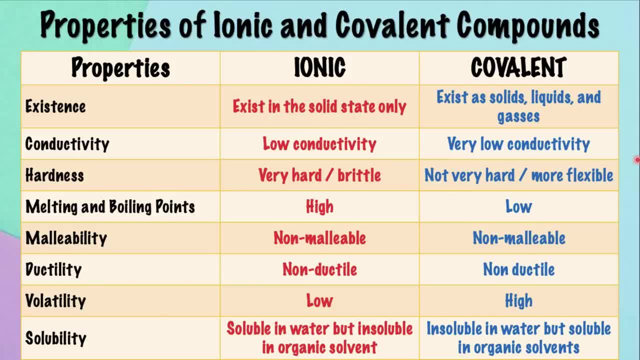 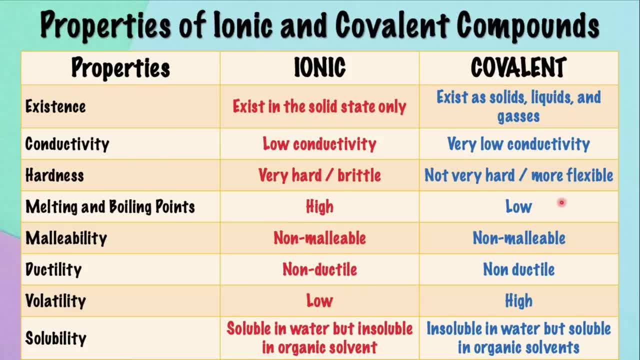